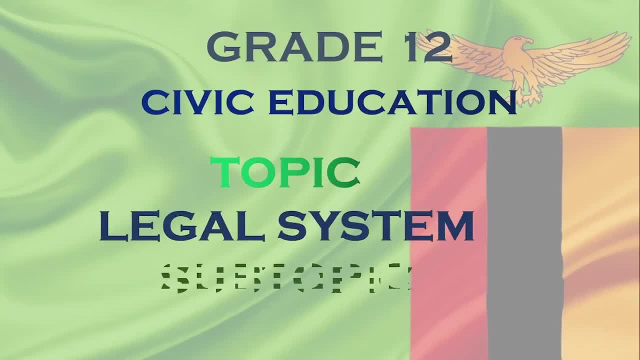 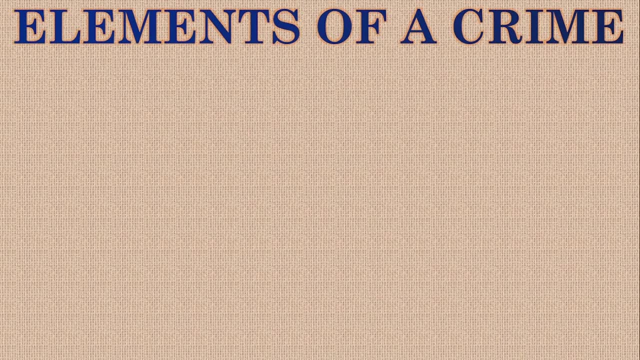 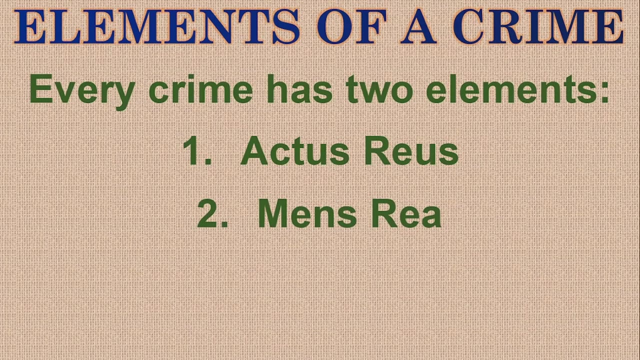 Welcome back to Civic Education Minds. I'm Teacher Kay. Today we are going to look at legal system and, in specific, we're going to look at the elements of a crime. Now, every crime has got two elements, and these elements are actors- rare- and men's rare. So let's look at these. 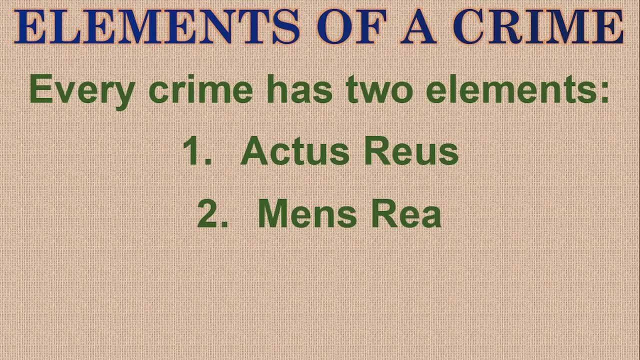 elements in details. but before we do that, I just want to emphasize that don't confuse the elements of a crime with the elements of a good legal system. These two are different Elements of a crime. there are two actors rare and men's rare. Let's look at these in details. 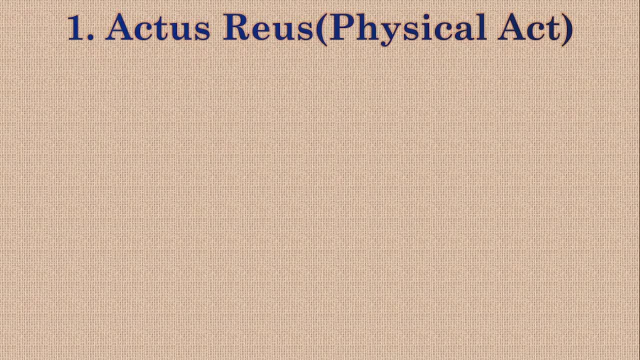 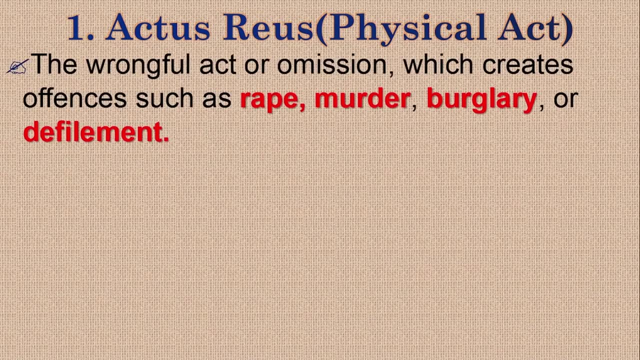 We have actors rare, the first one that we'll look at Now. these are latin terms and in english, actors rare means the physical act. What do we mean when we say actors rare? Here we are saying the wrongful act or omission which creates offenses such as. 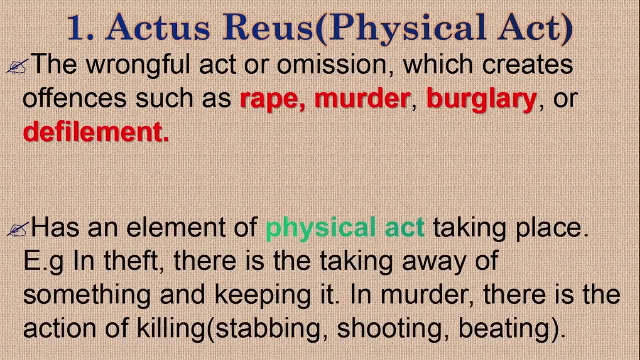 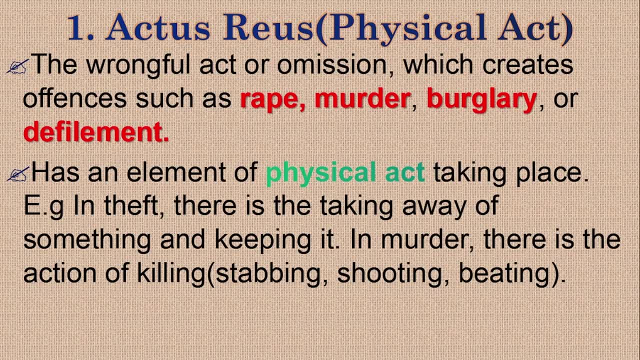 rape, murder, burglary or defilement. In other words, what we're trying to say is a crime has got an element of the physical act that takes place. For example, when we look at theft, there is the taking away of something and keeping it In. murder, there is the action of killing, So you can stab. 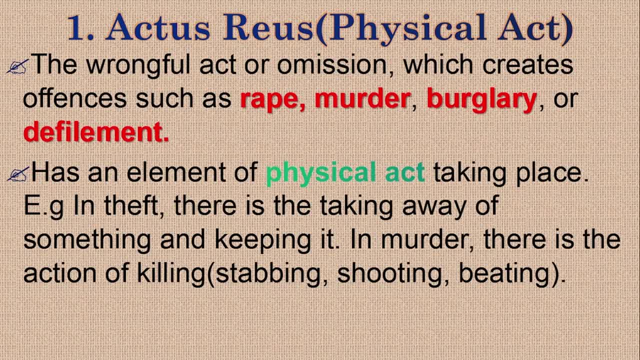 this person, you shoot this person, beat this person or any other way that you kill this person. So, in other words, what we're trying to say is a crime has got an element of the physical act that takes place. In other words, every crime has a physical act that is taking place, meaning someone. 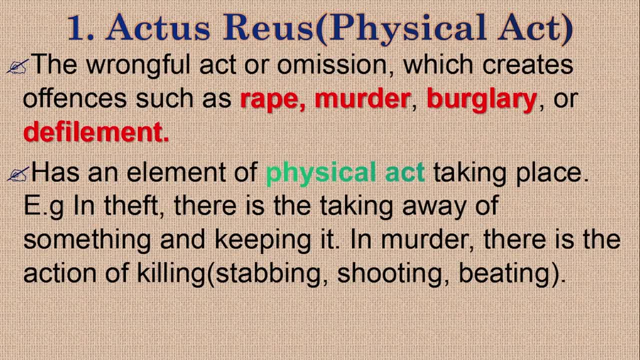 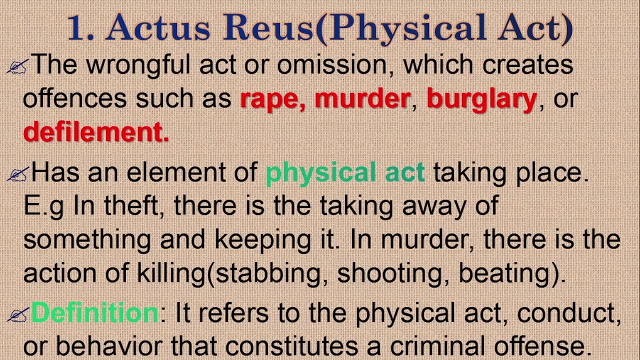 is performing an action, physically doing something. So actors rare just talks about the physical act that you perform when you're committing a crime. Now how can we define actors rare? if it comes in an exam We can say it refers to the physical act, conduct or behavior that constitutes a criminal. 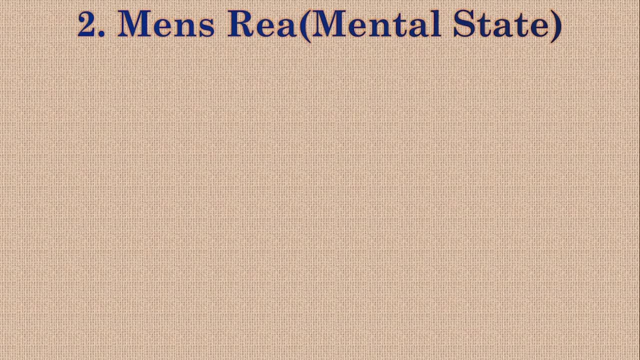 offense. Then we look at men's rare. Now, men's rare is a crime that takes place when a person is committing a crime. Now, men's rare is also a Latin term and in English it means mental state. So we're looking at the mental state. The first one: we're looking at the physical act that you do in committing. 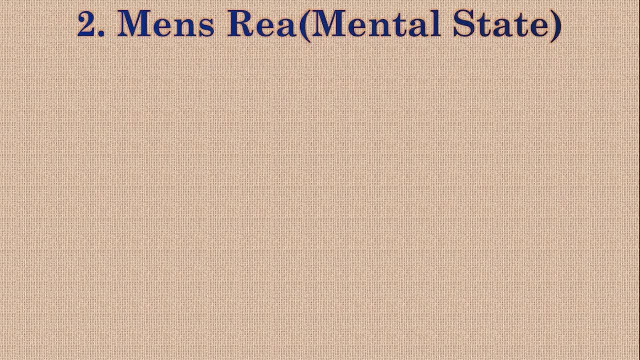 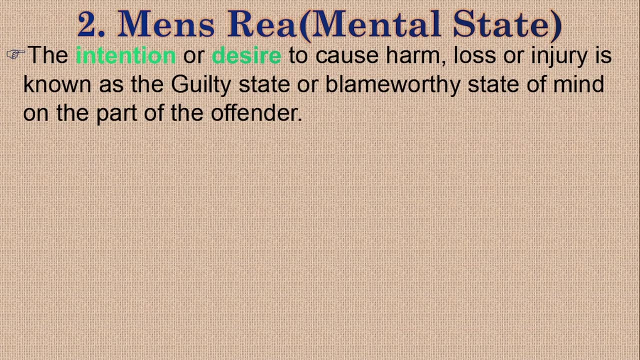 a crime. Here we're looking at the mental state, the mind of the person who was committing the crime. So here we're referring to the intention or the desire to cause harm, loss or injury on the victim, And when I say victim I'm referring to the person that was offended. We can also say it: 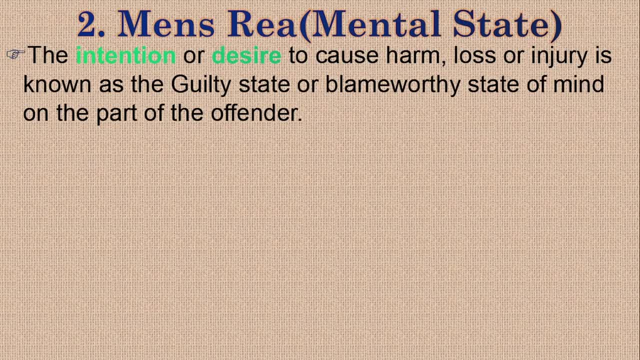 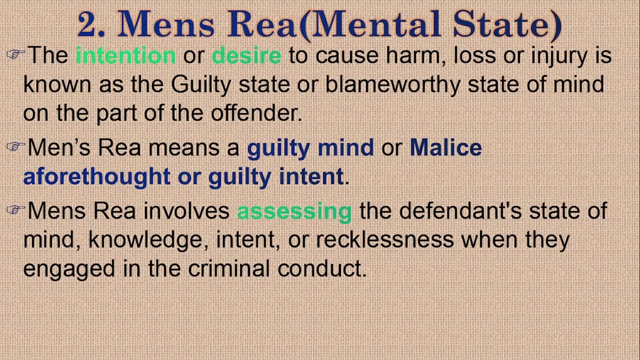 is the guilty state of the mind, the blame, with state of mind on the part of the offender. So, in other words, men's rare means a guilty mind, malice, awful thought or guilty intent. So men's rare involves assessing the defendant's state of mind, knowledge, intent or recklessness when they engaged. 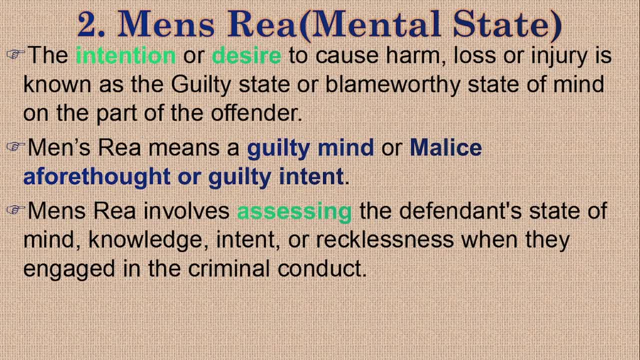 in the criminal conduct. When they were killing this person, did they know what they were doing? Were they aware that when I use a knife on this person, this is going to be the result? This is why you find that they have to look at the state of their mind, Because if you find, for example, someone who is mentally 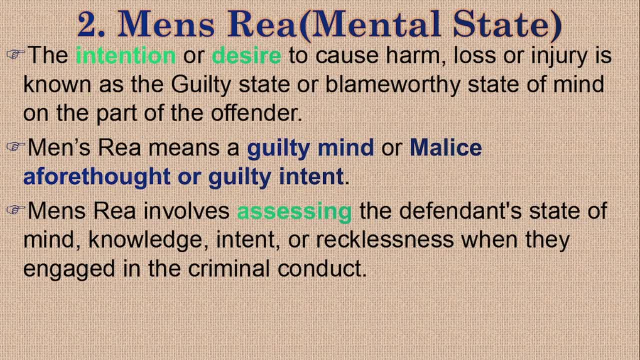 challenged. are they going to be aware, if they stab someone with a knife or if they stone someone, that this stone is going to cause harm to this person, or they just think that it is playing Same with a child? If a child gets a knife and playing with a brother stabs the brother or the 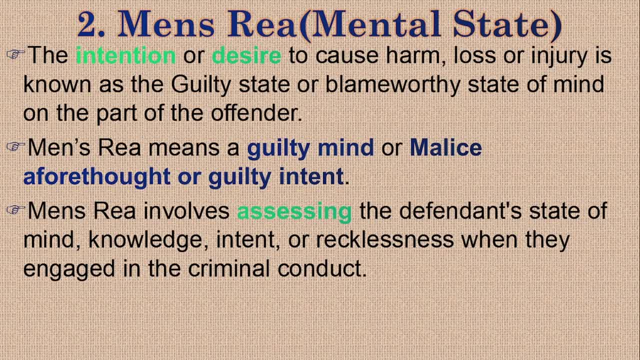 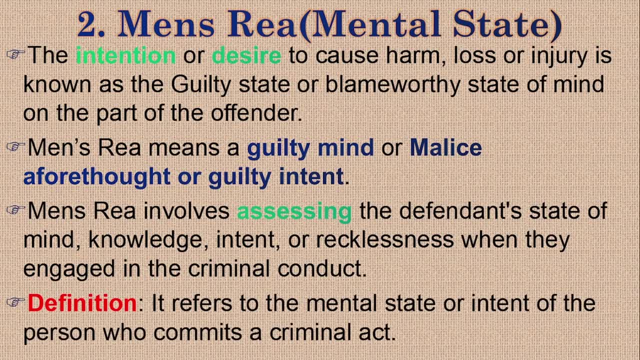 sister or the mother. they are going to be aware that this is going to cause harm to this person. They don't understand the harm that it is going to cause. So we're looking at the state of the mind and we can define it as the mental state or intent of the person who commits a criminal act. Let's 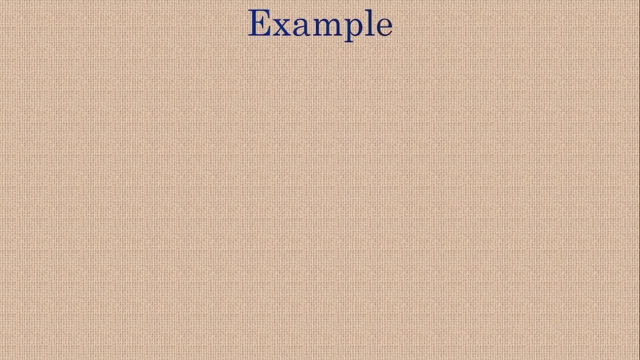 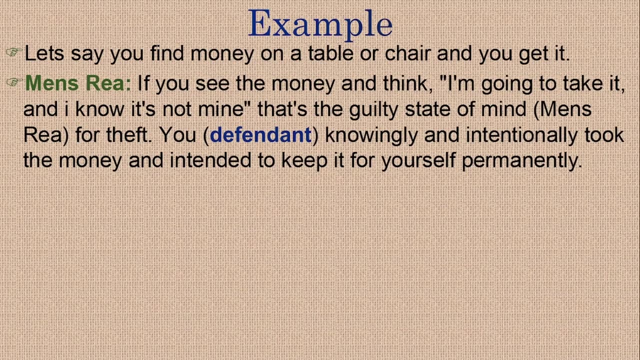 look at an example that will help us to understand these elements further. Let's say you find money on a table or chair and you get it In men's rare. we're saying, if you see the money and think I'm going to take it- and I know it's not mine- That's the guilty state. 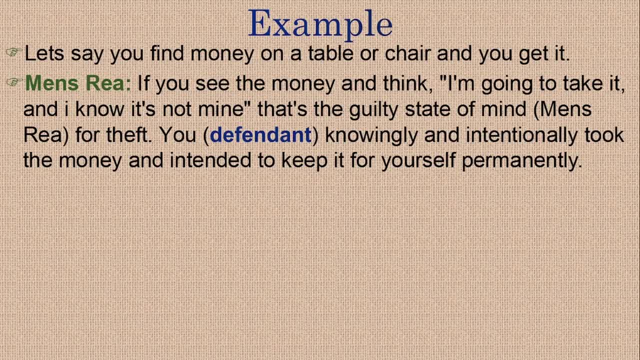 You know that the money is not yours, but you still decide to get the money. You knowingly and intentionally took the money and intended to keep the money for yourself permanently, without giving it back to the person that this money belongs to. Now, under the element of actus rare, the act of